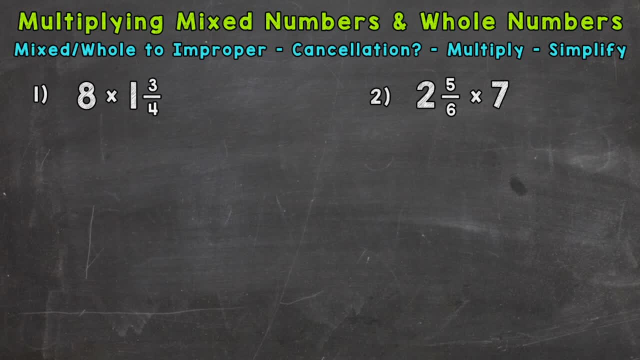 So for the whole number 8,, all we need to do for whole numbers is put them over 1 to change them to a fraction. So pretty simple. for whole numbers, Now, mixed numbers- we need to start at the bottom and work our way up. 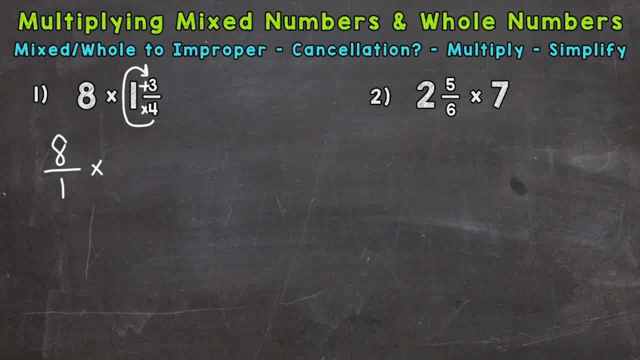 So we multiply and then add. We do 4 times: 1 is 4 plus 3 is 7.. We keep the denominator of 4 the same. So now we have the mixed number and whole number in fractional form. We have numerators and denominators. 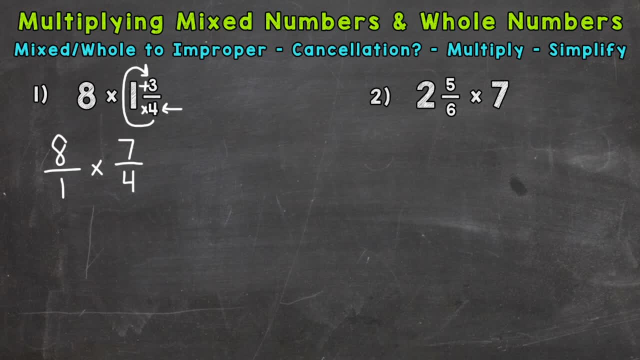 Now we can multiply straight across, But before doing so, you can check to see if you can use cancellation Cross-cancellation. This will help simplify the problem before we multiply, And in the case of number 1, we can use cross-cancellation. 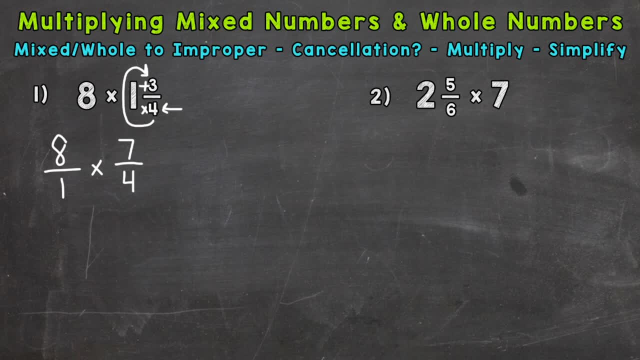 So you're looking for common factors between the numerators and denominators. So, for example, our 8 and 4 have a greatest common factor of 4. So we can divide both by 4.. 8 divided by 4 is 2.. 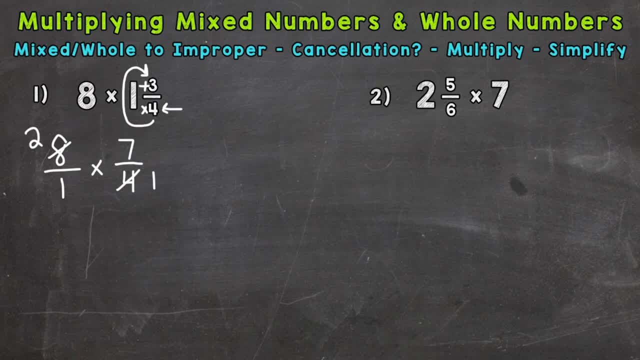 And 4 divided by 4 is 1.. So we now- We now have easier numbers to work with here, So we simplified the problem. You can think of it as simplifying the problem before you multiply. So 2 times 7 is 14.. 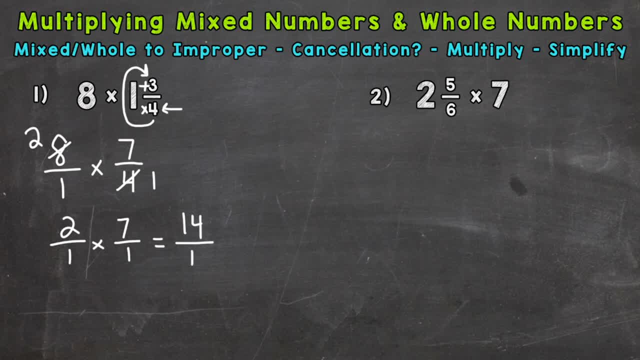 1 times 1 is 1.. So we end up with an improper fraction there: 14 over 1, which is just 14. We can write it as a whole number. Now I do want to mention when it comes to cross-cancellation. 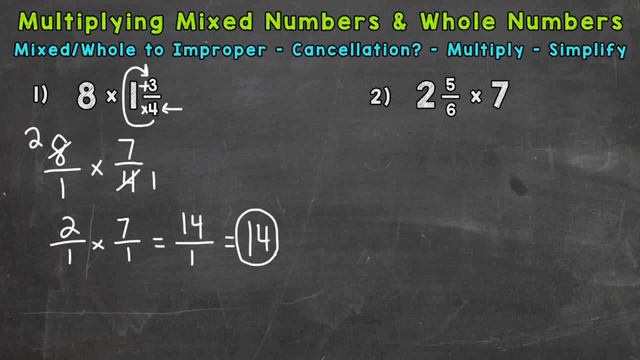 if you're not fully understanding that, I do have a video that goes into further detail. I'll drop that link down in the description. If you do not use cross-cancellation, you will still get to the correct answer. Let's actually do that. 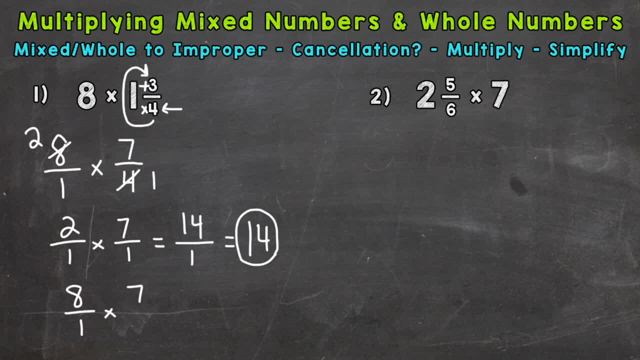 So we had 8 over 1 times 7 over 4.. So let's do it without cancellation and see what happens. 8 times 7 is 56.. 1 times 4 is 4.. So we got 56 over 4.. 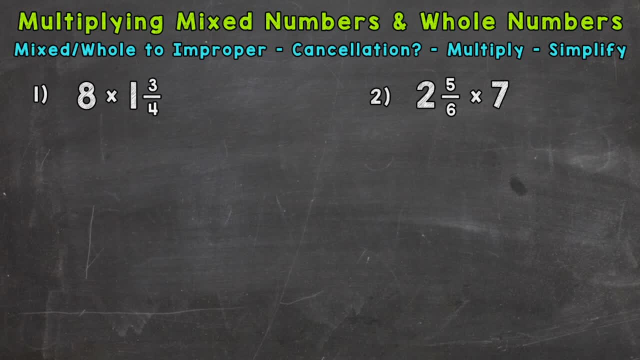 So for the whole number 8,, all we need to do for whole numbers is put them over 1 to change them to a fraction. So pretty simple. for whole numbers, Now, mixed numbers- we need to start at the bottom and work our way up. 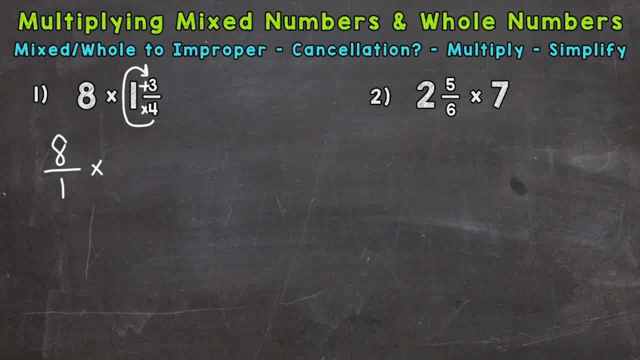 So we multiply and then add. We do 4 times: 1 is 4 plus 3 is 7.. We keep the denominator of 4 the same. So now we have the mixed number and whole number in fractional form. We have numerators and denominators. 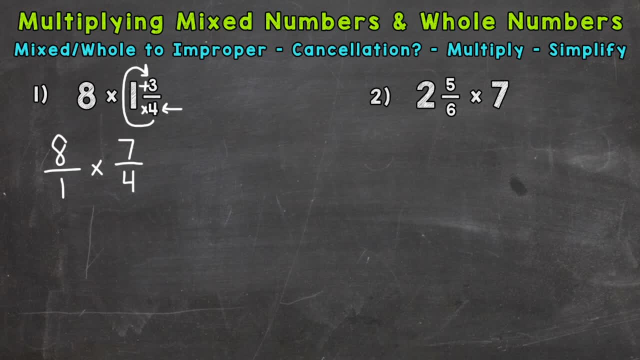 Now we can multiply straight across, But before doing so, you can check to see if you can use cancellation Cross-cancellation. This will help simplify the problem before we multiply, And in the case of number 1, we can use cross-cancellation. 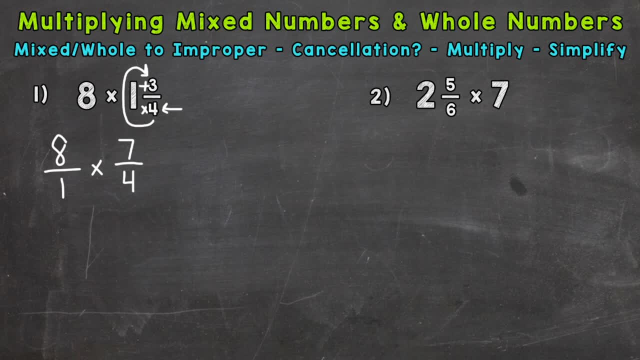 So you're looking for common factors between the numerators and denominators. So, for example, our 8 and 4 have a greatest common factor of 4. So we can divide both by 4.. 8 divided by 4 is 2.. 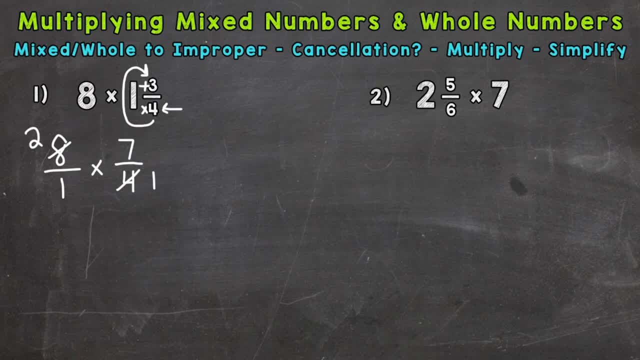 And 4 divided by 4 is 1.. So we now- We now have easier numbers to work with here, So we simplified the problem. You can think of it as simplifying the problem before you multiply. So 2 times 7 is 14.. 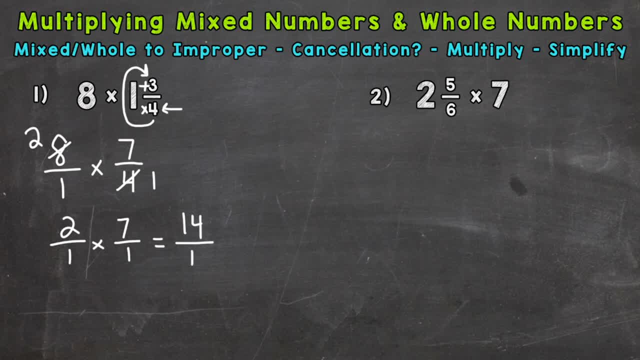 1 times 1 is 1.. So we end up with an improper fraction there: 14 over 1, which is just 14. We can write it as a whole number. Now I do want to mention when it comes to cross-cancellation. 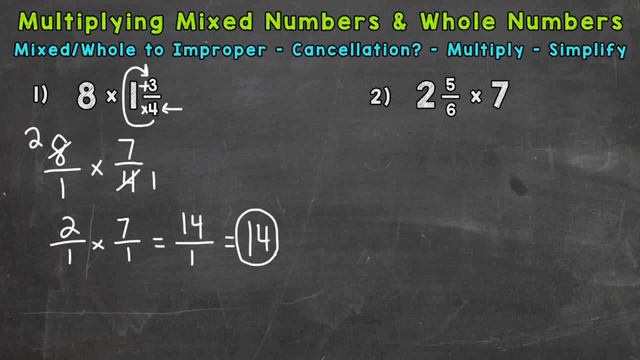 if you're not fully understanding that, I do have a video that goes into further detail. I'll drop that link down in the description. If you do not use cross-cancellation, you will still get to the correct answer. Let's actually do that. 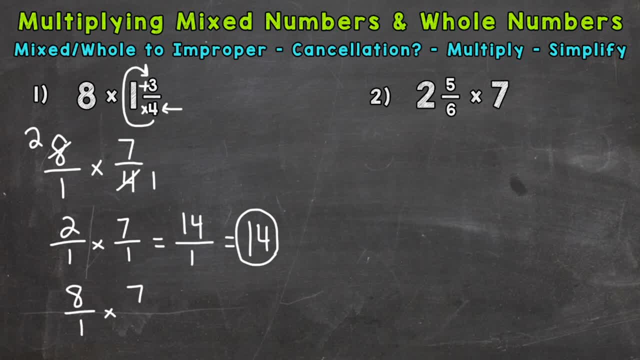 So we had 8 over 1 times 7 over 4.. So let's do it without cancellation and see what happens. 8 times 7 is 56.. 1 times 4 is 4.. So we got 56 over 4.. 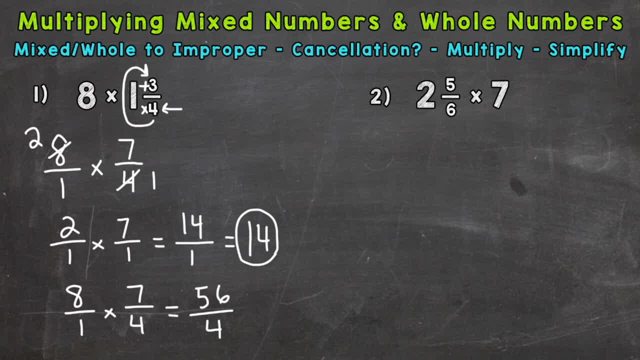 Instead of 14 over 1.. But we need to simplify here. We have an improper fraction. We need to convert this to a mixed number, or maybe it works out to a whole number. So we do that by dividing the numerator 56, by 4.. 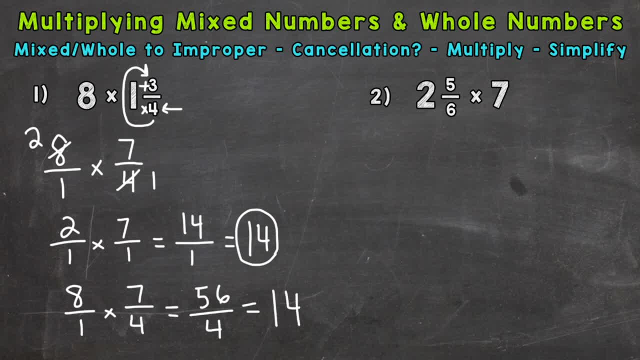 So 56 divided by 4 does work out to be 14.. So you can see that we got the same answer On to number 2, where we have 2 and 5 sixths Times 7.. So again, first thing we need to do is change or convert our mixed numbers and whole numbers to fractions. 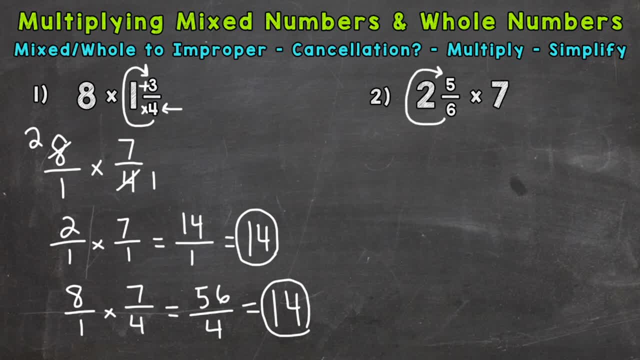 So let's do our mixed number here. Start at the bottom, Multiply and add. So 6 times 2 is 12. Plus 5 is 17.. Keep the denominator of 6, the same Times, Remember, for any whole numbers. 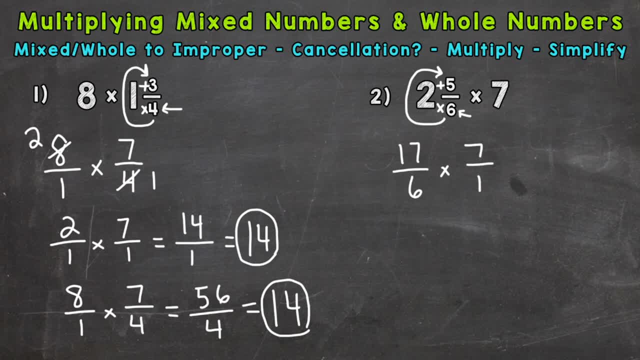 8 over 1 to put it in fractional form. So 7 over 1 there. Now let's see if we can use any cancellation in order to simplify this problem. before multiplying, So check to see if we have any common factors between the numerators and denominators other than 1.. 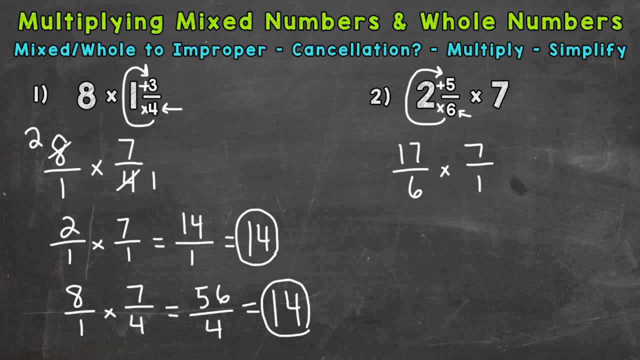 But in the case of number 2, the only common factors we have between 6 and 7, 17 and 1 is 1.. So we cannot use cancellation. So we go right to multiplying straight across And we'll start with 17 times 7, which we can come to the side to solve. 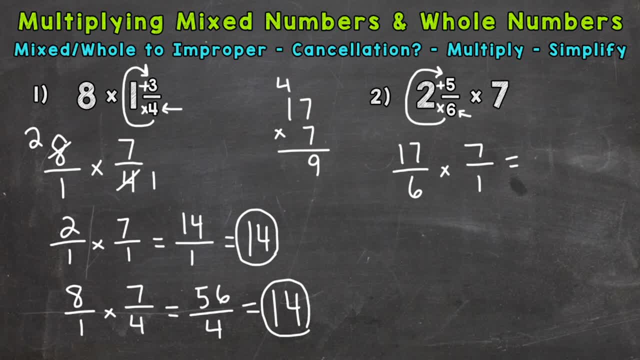 7 times 7, 49.. 7 times 1 is 7.. Plus 4, 11.. So we get 119.. 6 times 1 is 6.. So we end up with an improper fraction which we need to. 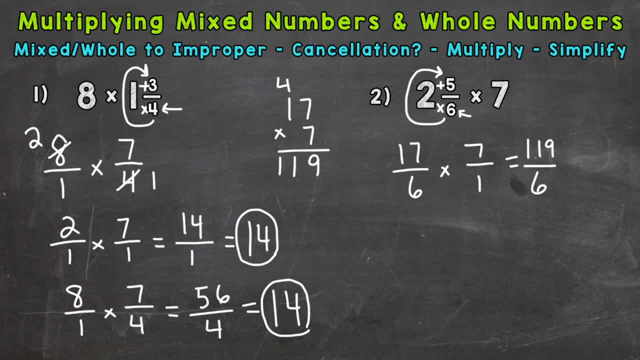 Change to a mixed number And then see if we can simplify any further if we have any fractions involved after we do that. So it's either going to work out to a whole number like number 1. Or if we have a remainder, it's going to work out to be a mixed number. 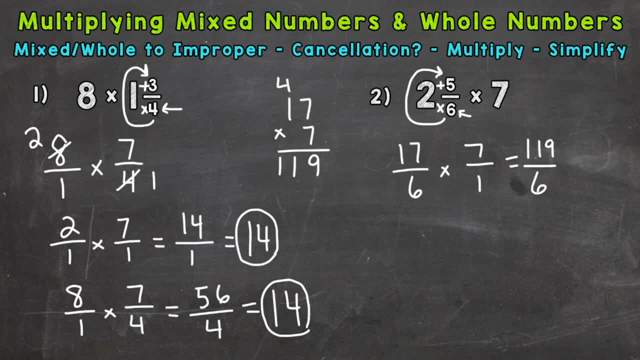 So we need to do 119 divided by 6.. So let's come down here: 119 divided by 6.. So we'll start with Start with 11 divided by 6, which is 1.. 1 times 6 is 6.. 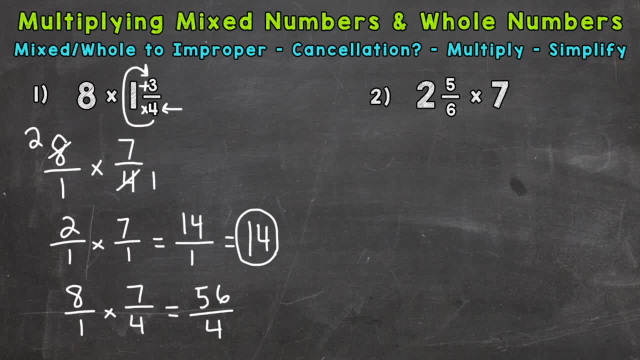 Instead of 14 over 1.. But we need to simplify here. We have an improper fraction. We need to convert this to a mixed number, or maybe it works out to a whole number. So we do that by dividing the numerator 56 by 4.. 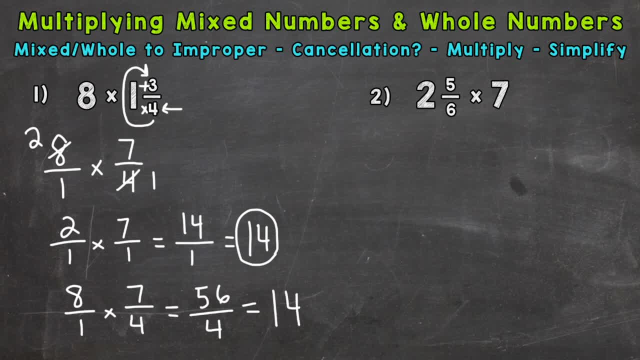 So 56 divided by 4 does work out to be 14.. So you can see that we got the same answer On to number 2, where we have 2 and 5 sixths. 2 and 5 sixths. 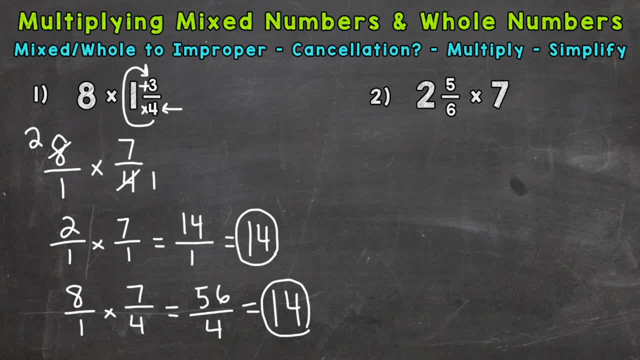 Times 7.. So again, first thing we need to do is change or convert our mixed numbers and whole numbers to fractions. So let's do our mixed number here, Start at the bottom, Multiply and add. So 6 times 2 is 12.. 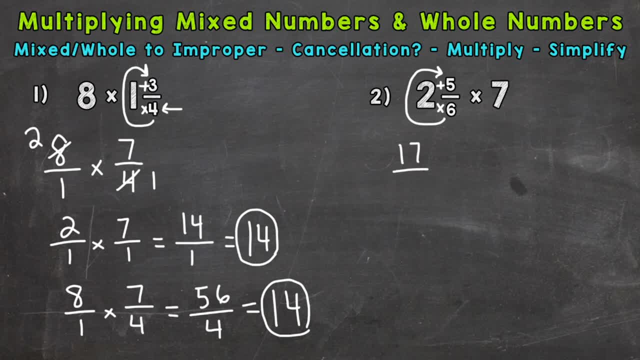 Plus 5 is 17.. Keep the denominator of 6, the same Times Remember for any whole numbers. we can just put it over and over again: 7 over 1 to put it in fractional form. So 7 over 1 there. 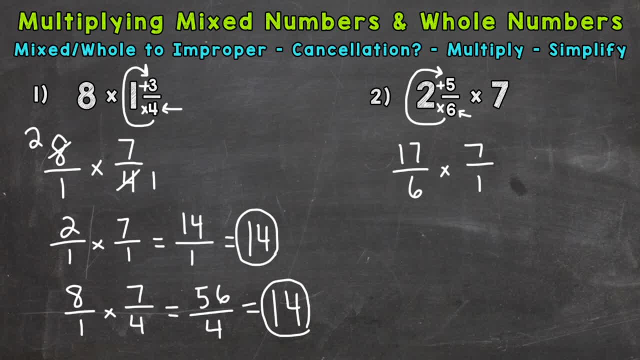 Now let's see if we can use any cancellation in order to simplify this problem before multiplying. So check to see if we have any common factors between the numerators and denominators other than 1.. But in the case of number 2,, 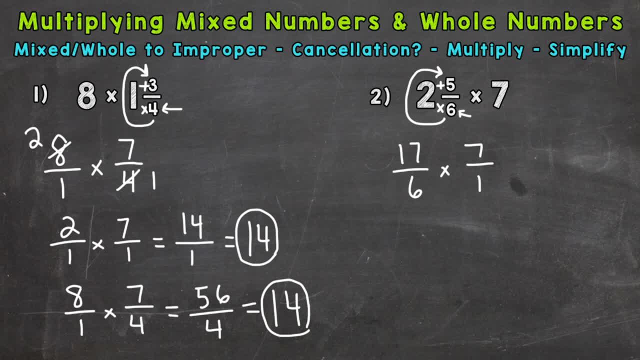 the only common factors we have between you know 6 and 7,, 17 and 1 is 1.. So we cannot use cancellations. So we go right to multiplying straight across And we'll start with 17 times 7,. 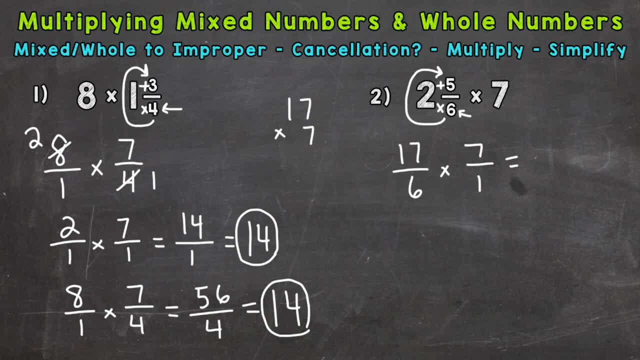 which we can come to the side to solve 7 times 7, 49.. 7 times 1 is 7.. Plus 4, 11.. So we get 119.. 6 times 1 is 6.. So we end up with an improper fraction. 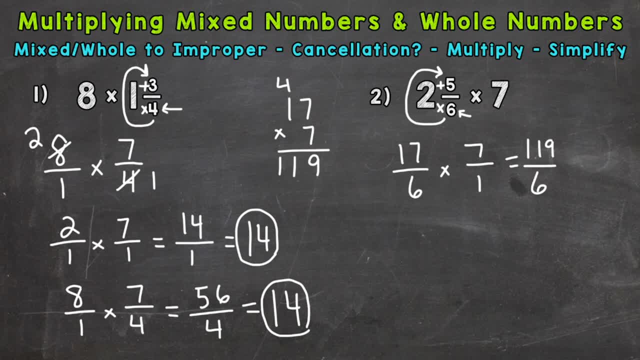 which we need to change to a mixed number and then see if we can simplify any further if we have any fractions involved after we do that. So it's either going to work out to a whole number like number 1, or if we have a remainder.